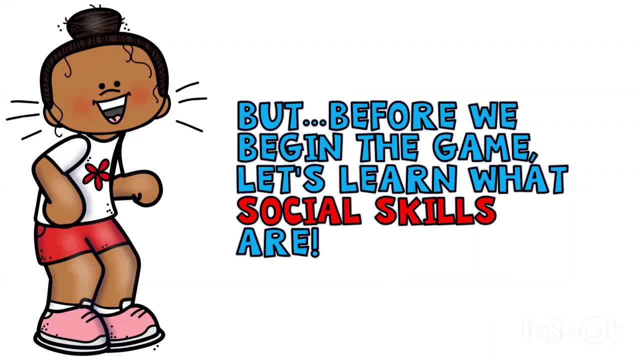 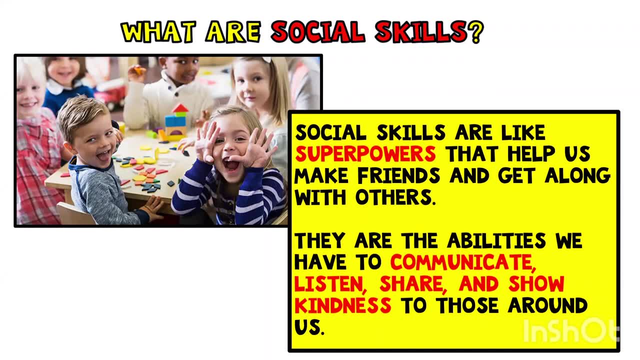 let's learn what social skills are. So what are social skills? Social skills are like superpowers that help us make friends and get along with others. They are the abilities we have to communicate, listen, share and show kindness to those around us. Why are social skills important? 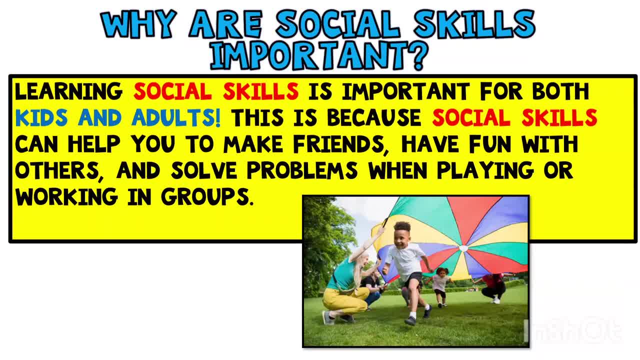 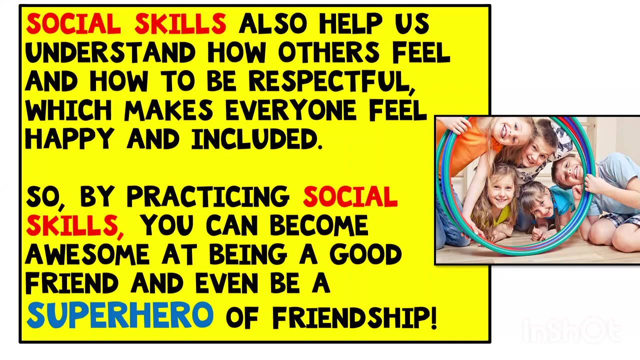 Learning social skills is important for both kids and adults. This is because social skills can help you to make friends, have fun with others and solve problems when playing or working in groups. Social skills also help us understand how others feel and how to be respectful. 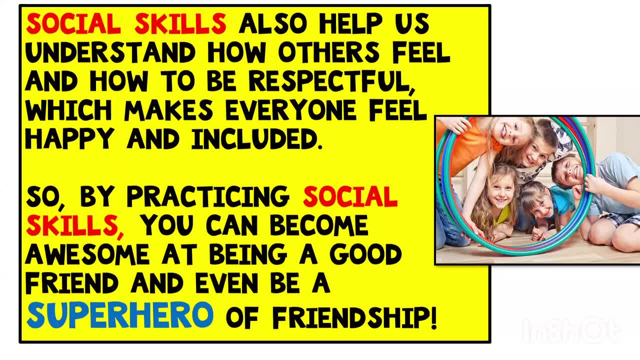 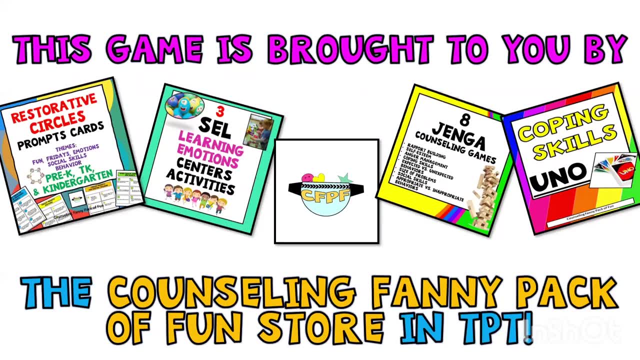 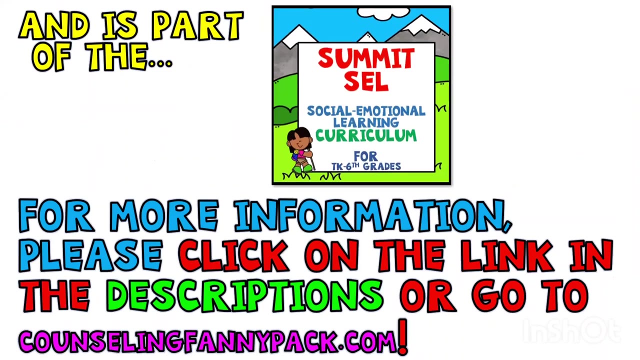 which makes everyone feel happy and included. So by practicing social skills, you can become awesome at being a good friend and even being a superhero of friendship. This game is brought to you by Counseling Fannie Pack of Fun and Teachers Pay Teachers and is part of the Summit SEL Social Emotional Learning Curriculum For. 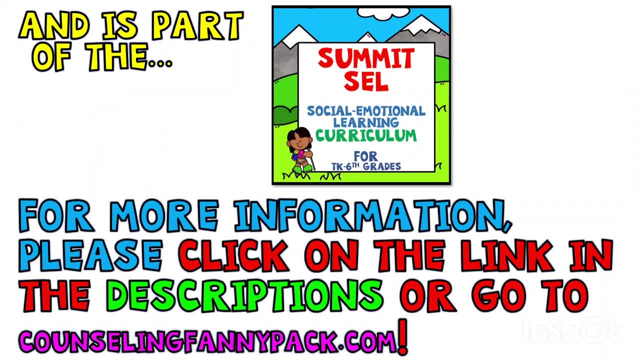 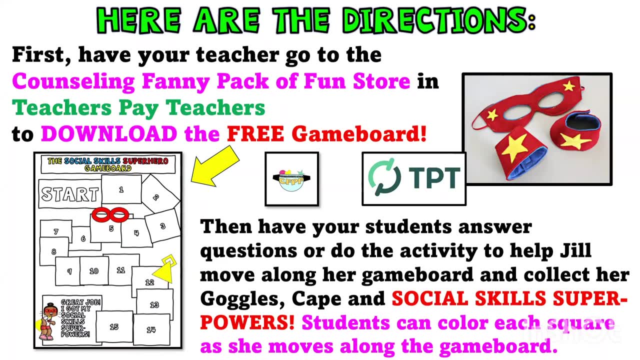 teachers who want to learn more about social skills, please visit the link in the description or go to counselingfanniepackcom. Here are the directions. First, have your teacher go to the Counseling Fannie Pack of Fun store and Teachers Pay Teachers to download the free game board. 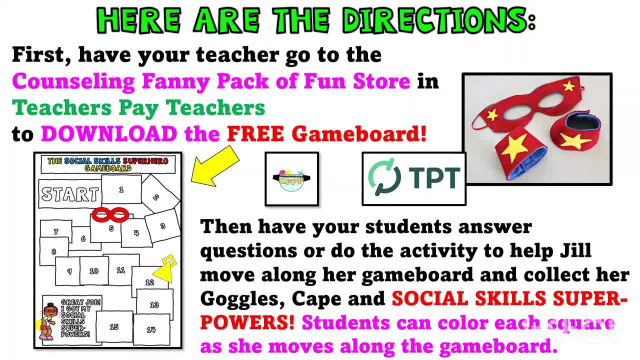 Then have your students answer questions or do the activity to help Jill move along her game board And collect her goggles, cape and social skills superpowers. Students can color each square as she moves along the game board, or just put an X, whatever you like, Be aware that you may. 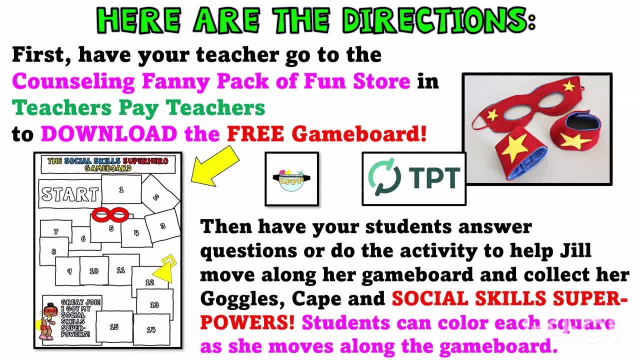 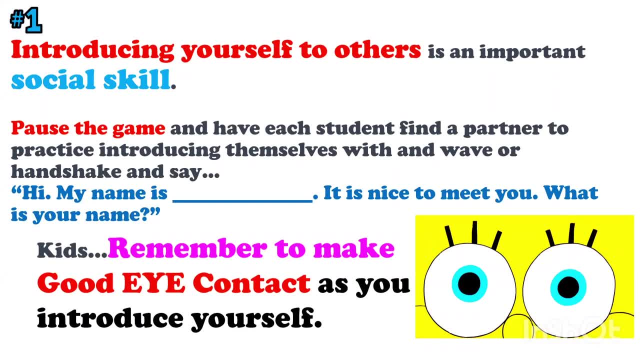 get out of your chair to play some of the activities or answer some of the questions. Square number one: Introducing yourself to others is an important social skill. Pause the game and have each student find a partner quickly to practice introducing themselves with and wave or handshake while saying: Hi, my name is blank. It's nice to meet you. What is your? 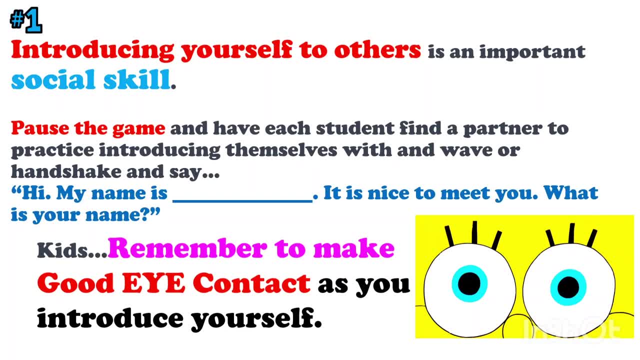 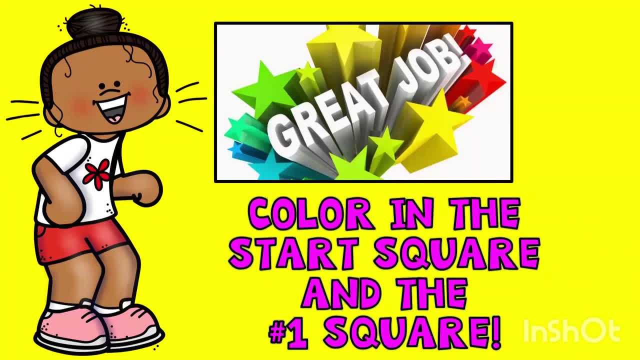 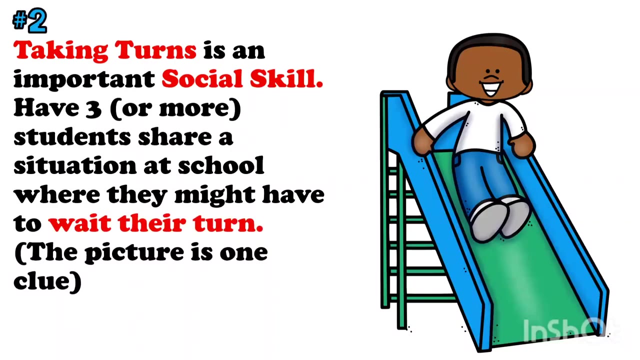 name Kids. remember to make good eye contact as you introduce yourself. Now pause the game. Great job everyone. Now you can color in the start square and the number one square. Let's go on to question number two, or activity Taking turns is an important social skill. 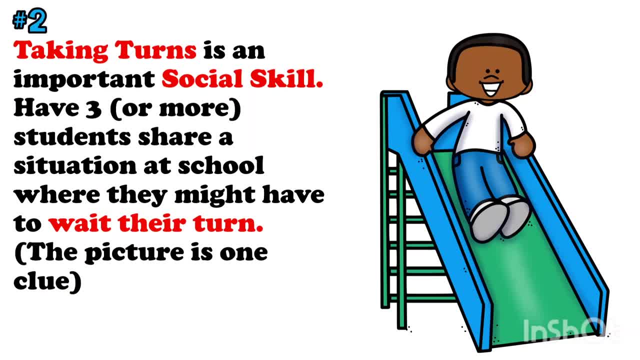 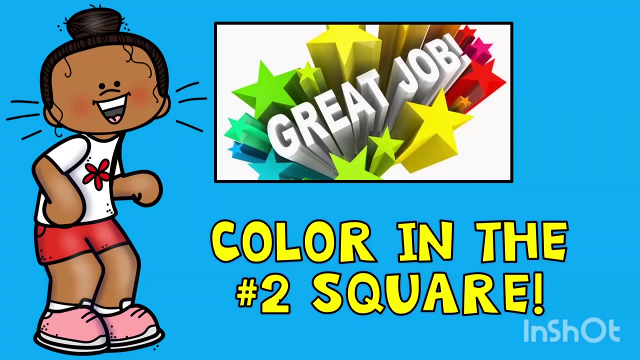 Have three or more, if you like. students share a situation at school where they might have to wait their turn. The picture is one clue. See if you can think of some other ones. Great job: color in the number two square: Teachers or counselors, remember. 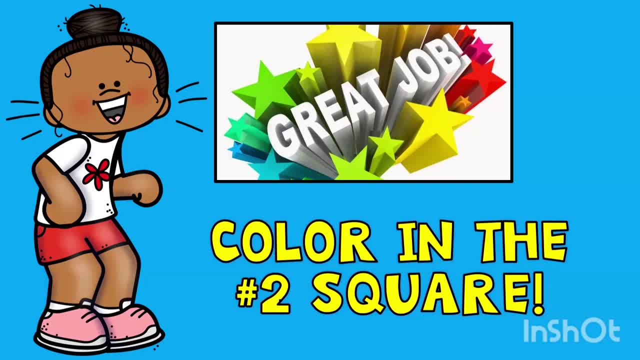 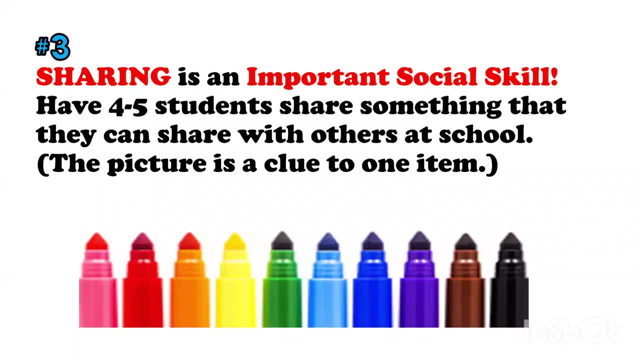 you can pause the game at any time. if you think that answering questions for your students might take a little bit longer than about 10 seconds, All right, let's go to number three. Sharing is an important social skill. Have four to five students share something. 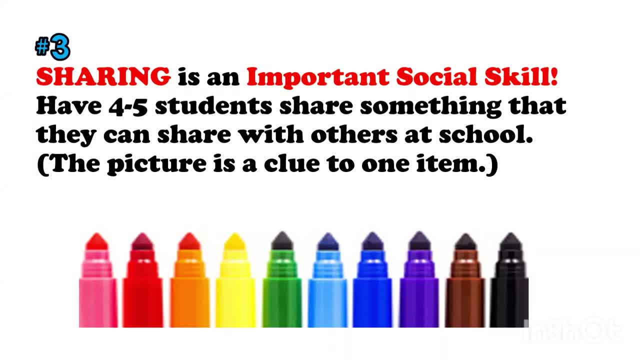 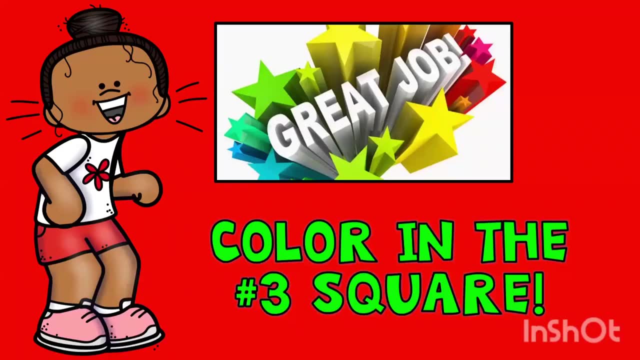 that they can share with others at school. The picture is a clue to one item. See if you can think of some other things that would be great to share at school, or that even you have to share. Great job. color in the number three square. 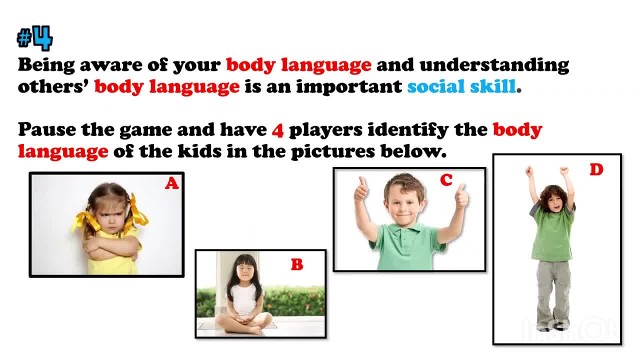 Number four: being aware of your body language and understanding others' body language is an important social skill. Pause the game and have four players identify the body language of the kids in the pictures below. Are they happy, sad, excited, calm, nervous, scared? 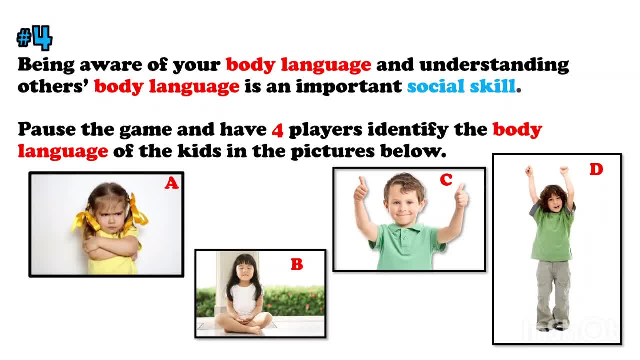 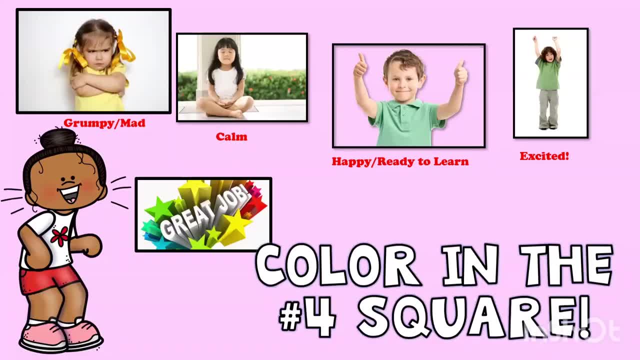 What do you think? I'm sure you're excited. I'm sure you're excited. What do you think If you said girl number one looked grumpy or mad? you are right. Girl number two is calm. Boy number three is happy and ready to learn. 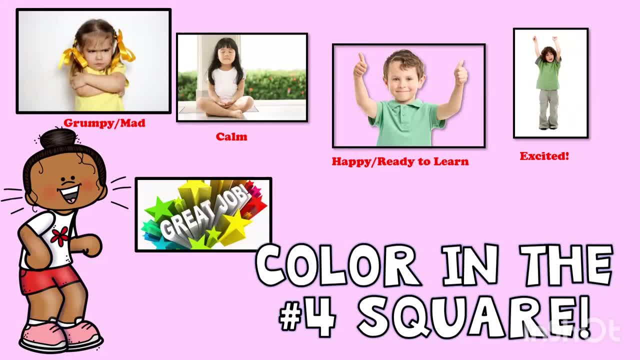 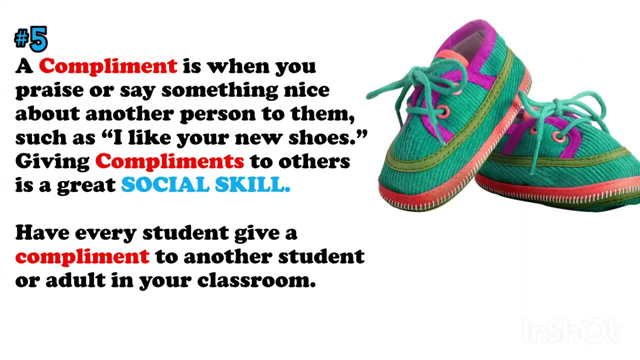 And boy number four looks pretty excited, But if you had something to say that was similar I'm sure you were right. You're in the number four, square Number five. a compliment is when you praise or say something nice about another person to them, such as I like your new shoes. 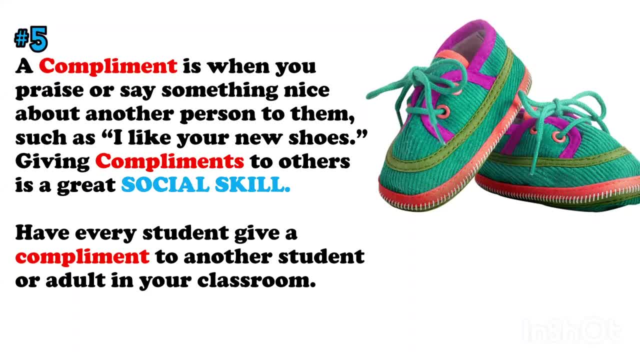 Giving compliments to others is a great social skill. Have every student give a compliment to another student or adult in your classroom. Feel free to walk around a little bit. It kind of makes things fun. Or you can stand in a circle and just turn to the person next to you and think of something. 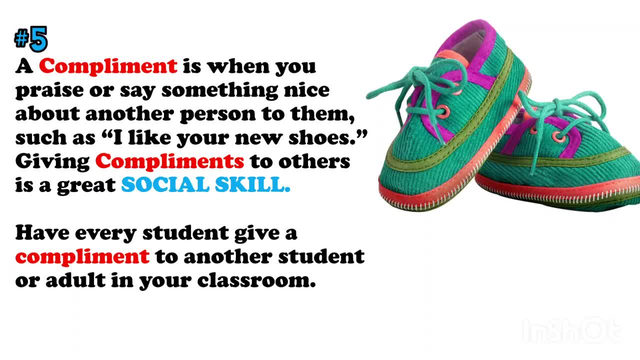 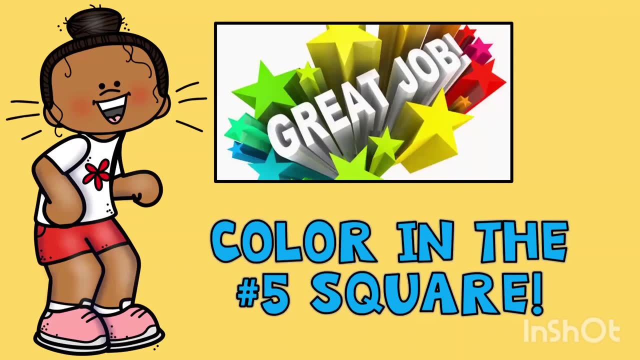 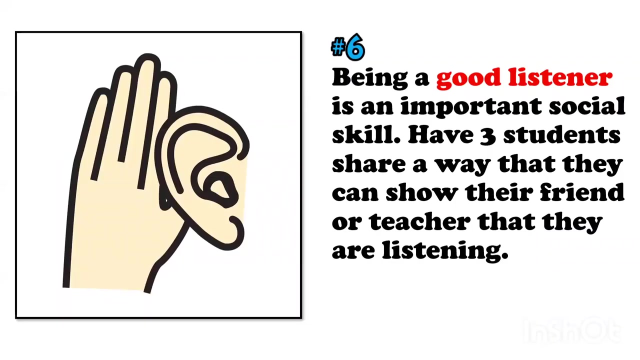 nice to say: I like your shoes, You have a great haircut, You're a really nice person Or you're super funny. Okay, Okay, Great job. everyone. Color in the number five: square. Pause the game if you need more time for coloring. 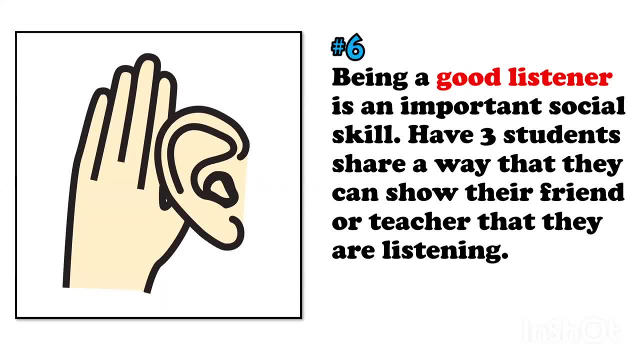 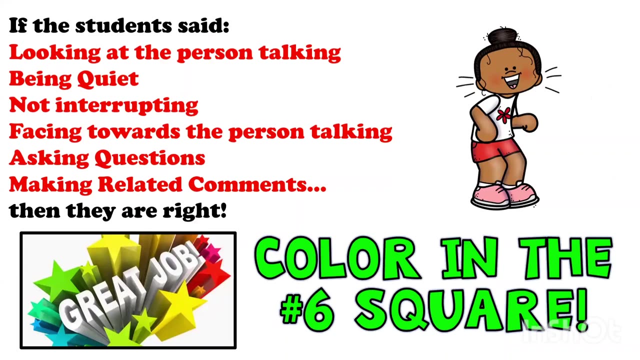 Number six: being a good listener is an important social skill. Have three students share a way that they can show their friend or teacher that they're listening If the students said something like looking at the person talking, being quiet, such as not interrupting, facing towards the person talking. so we don't want to put our back. 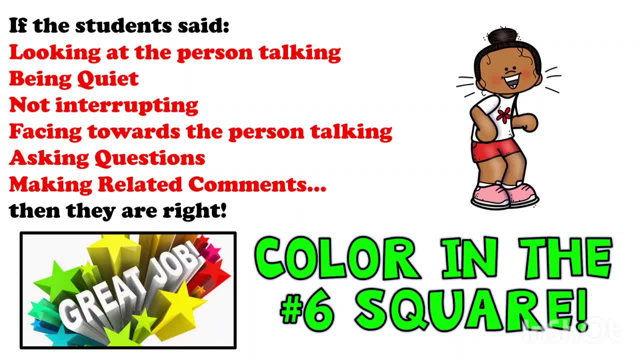 to them. if they're talking to us, right, That might make them think we're not listening. Asking questions: that's a good way to show somebody that you're paying attention to what they're saying and also making related comments. So if your friend is saying: I got a new puppy, asking questions might be: what color is your? 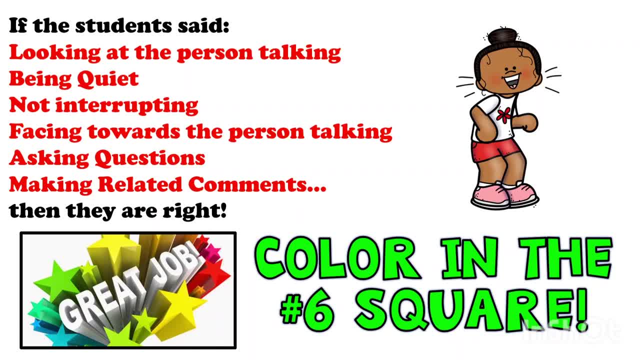 puppy. What's your puppy's name Making a related comment would be: oh wow, I really like dogs. I'm so happy for you that you got a new puppy. Okay, Let's move on to number six. Color in the number six square. 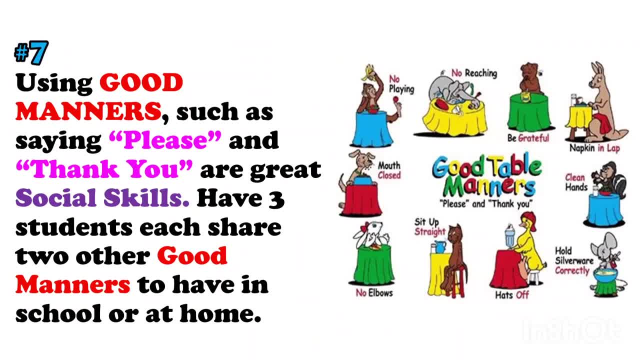 Number seven: using good manners such as saying please and thank you are great social skills. Have three students each share two other good manners to have in school or at home. Here's some examples of good table manners that you can pause. Pause the game. 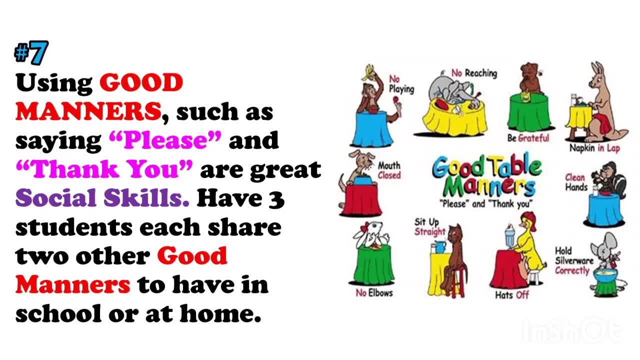 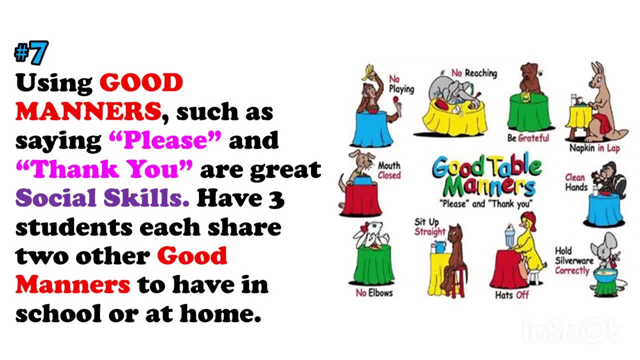 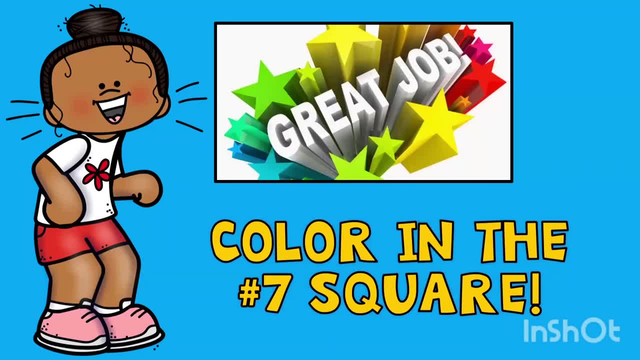 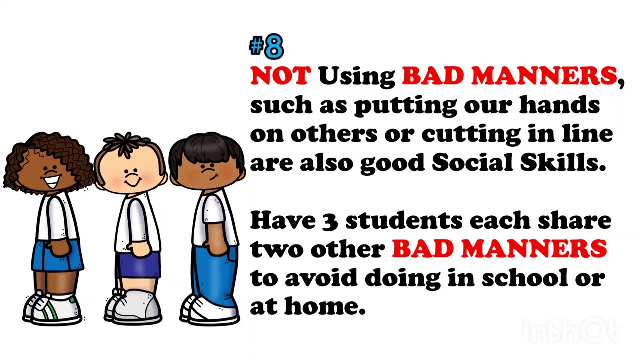 If you can think of some other ones, especially at school, that would be great. Pause the game. I'm sure everyone thought of great manners. Color in the number seven, square Number eight: not using bad manners such as putting a dog on the table. 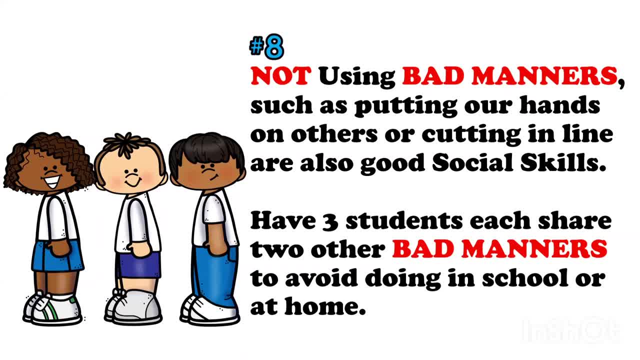 You'll notice that there are other bad manners that are in class, Like putting our hands on people throughout the class, Like putting our hands on people first, Putting our hands on people on their afternoon when they come into class And complained about the dog afterwards. 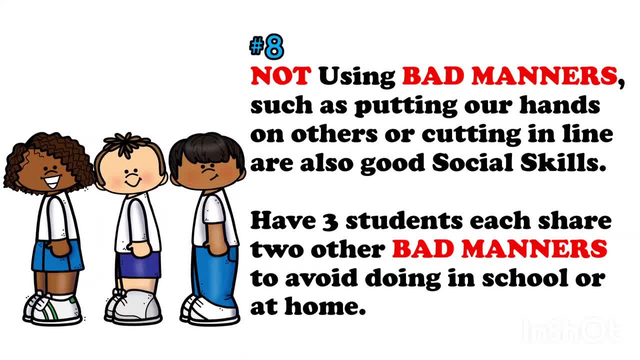 And Normally you don't cut your hands while you cut the dog: Cutting some new ones alive, Cutting some old ones alive, Cutting an old one alive. They may die to the cu papers and are even better than to cut up aons of yours. 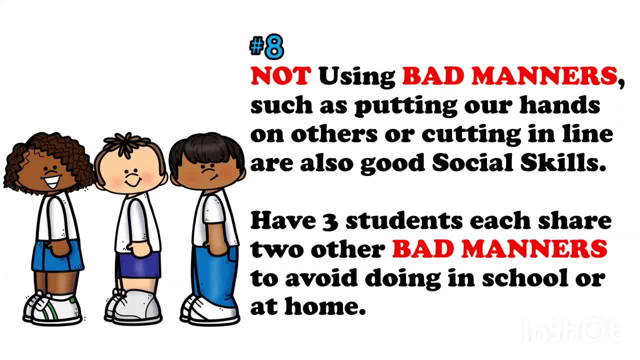 Playing soccer balls before work A or after work doesn't mean anybody cheers for you on that day. Very good�ään, hand over another trained person lunch maybe, or something like that is good to get Aon a pick your way in 되지. 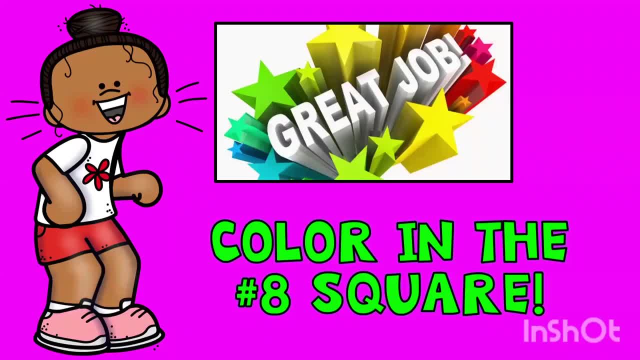 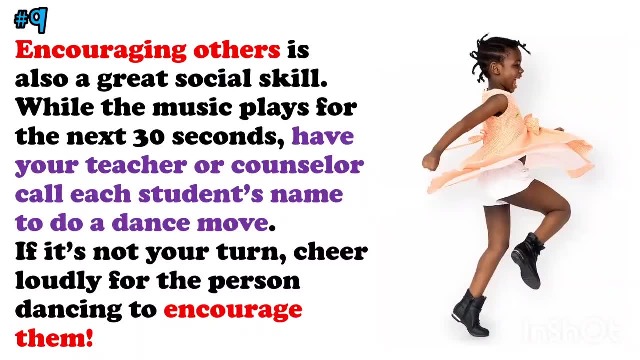 Dis 여기서 angry parents. don't look at this question yet. Pause the game. Great job: Color in the number eight square Number nine. Encouraging others is also a great social skill. While the music plays for the next 30 seconds. 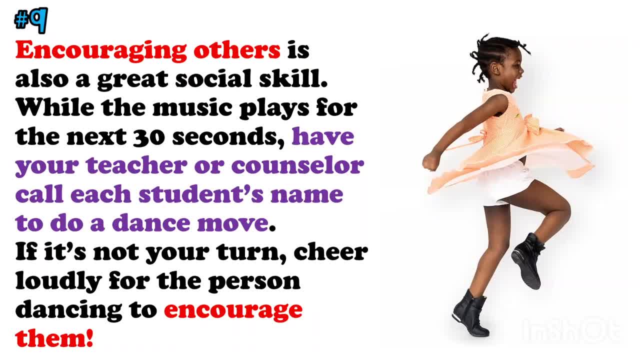 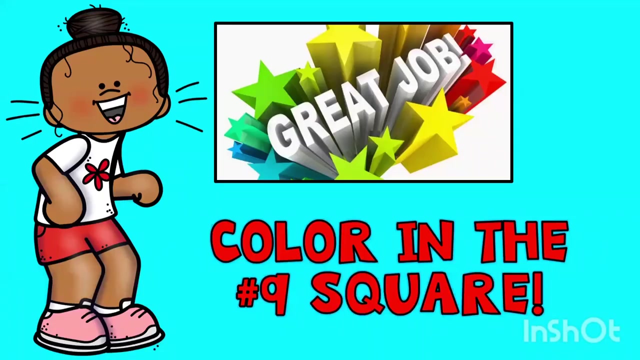 have your teacher or counselor call each student's name to do a dance move. If it's not your turn, practice cheering loudly for the person who is dancing to encourage them Ready and go. Awesome dance moves, guys. Great job. Color in the number nine square. 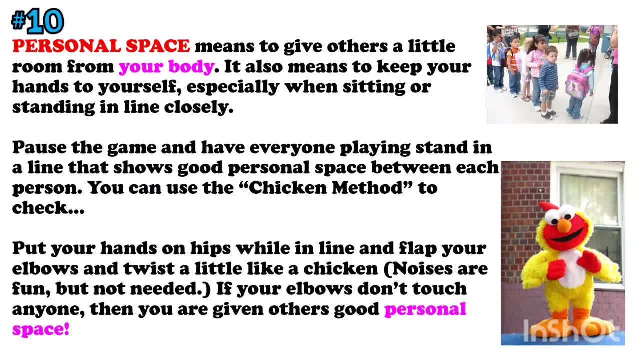 Number 10.. Personal space means to give others a little room from your body. It also means Keep your hands to yourself, especially when sitting or standing in line closely. Pause the game and have everyone playing. stand in a line that shows good personal space between each person. 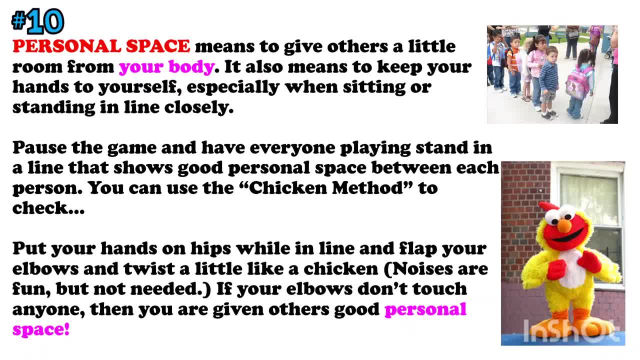 You can use the chicken method to check. To do the chicken method, put your hands on your hips or sides, just like the picture of Elmo, And flap a little bit and do a little twist. If you're not touching anybody, then you're giving others good personal space. 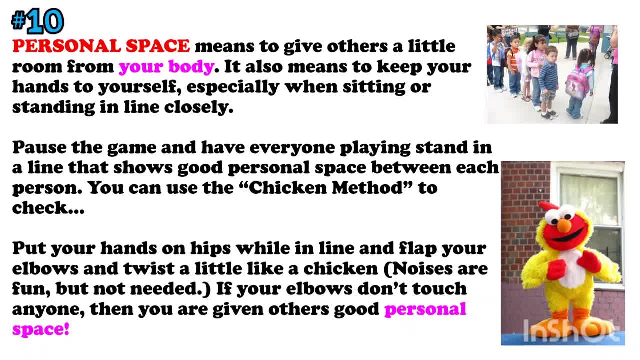 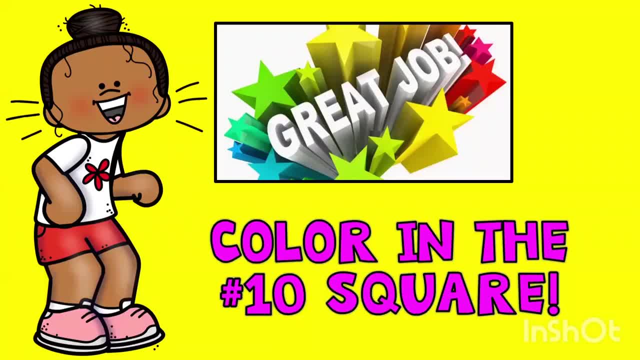 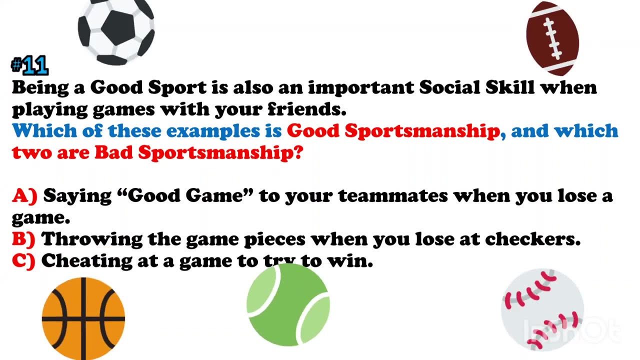 Noises are fun but not needed. Great job. Color in the number 10, square Number 11.. Being a good sport is also an important social skill when playing games with your friends. Which of these examples is good sportsmanship and which two are bad sportsmanship? 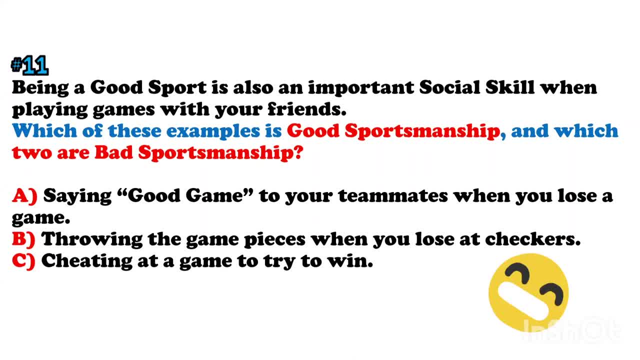 Saying good game to your teammates when you lose a game. Throwing the game pieces when you lose a game. Throwing the game pieces when you lose a game Number 11.. lose at checkers and see cheating at a game to try to win a was good. 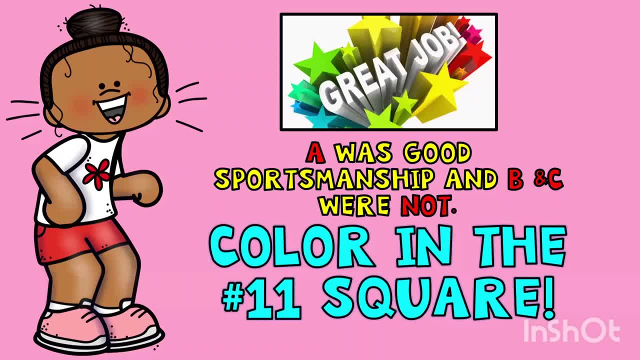 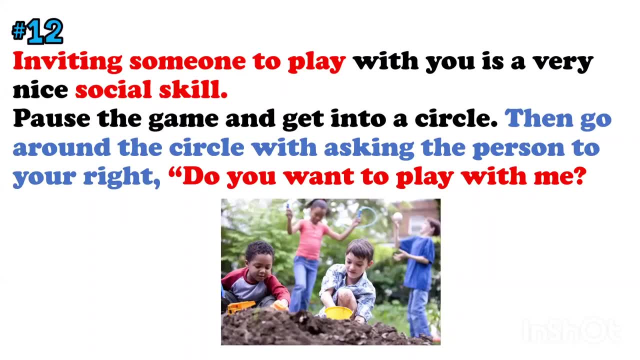 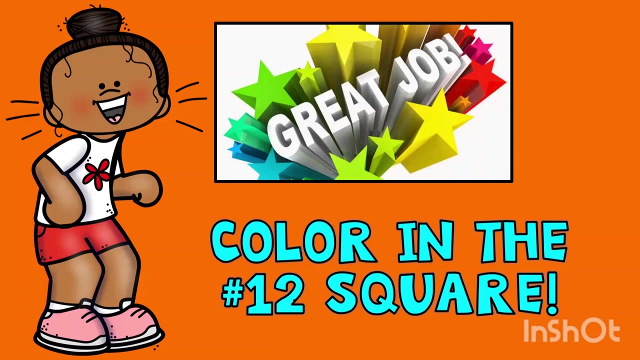 sportsmanship and B and C were not. color in the number. 11. square number 12: inviting someone to play with you is a very nice social skill. pause the game and get into a circle. then go around the circle with asking the person to your right. do you want to play with me? pause the game. great job. color in the number. 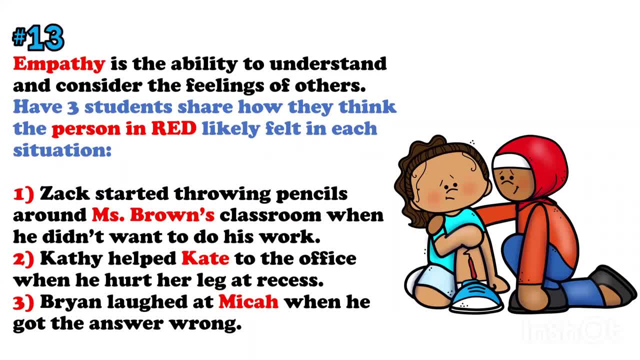 12 square. number 13: empathy is the ability to understand and consider the feelings of others. have three students share how they think the person in red and the sentences below likely felt in each situation. number one: Zack started throwing pencils around mrs Brown's classroom when he didn't want to. 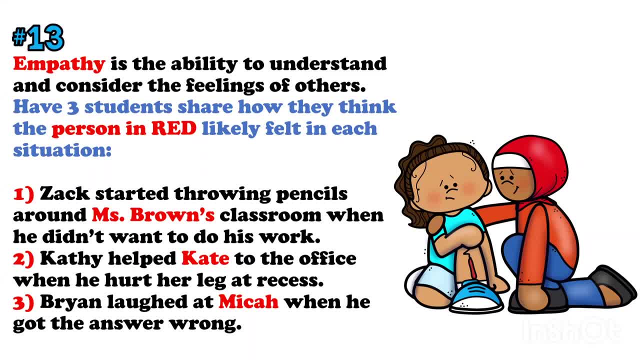 do his work. how did mrs Brown feel? number two: Kathy helped Kate to the office when she hurt her leg at recess. how did Kate feel that somebody was helping her? number three: Brian laughed at Micah when he got the answer wrong. how did Micah feel in that situation if? 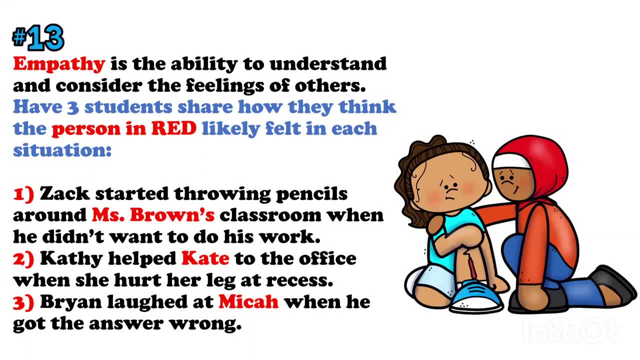 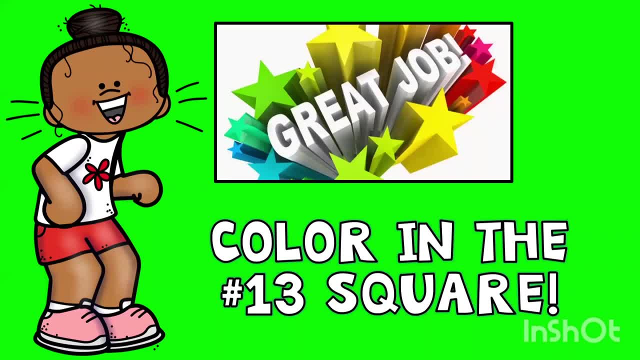 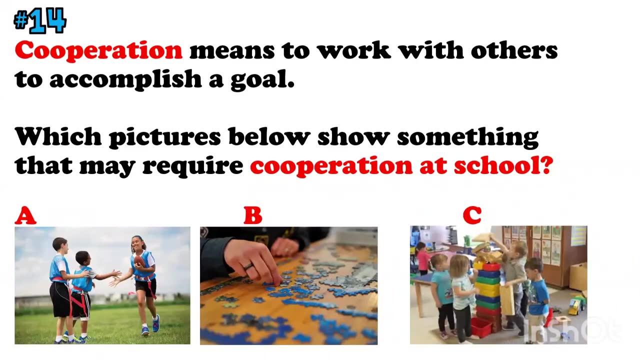 you knew the answers, then you might know how to give others empathy. you so great job. color in the number 13: square. Riley has her cape and goggles by now. I'm so excited for her. I hope she makes it to the end to get her superpower. number 14: cooperation means to work with others to accomplish a goal. 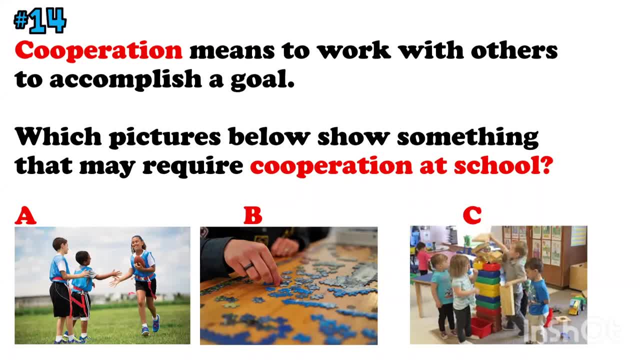 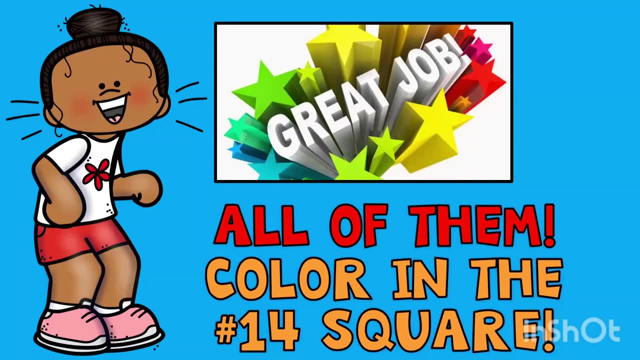 which pictures below show something that may require cooperation. that school- a, B or C- all of them- puzzles. you can work by yourself or you could work with somebody else to solve them: building towers and Legos. that could be a group activity, and playing sports is usually a group activity, especially when there's a 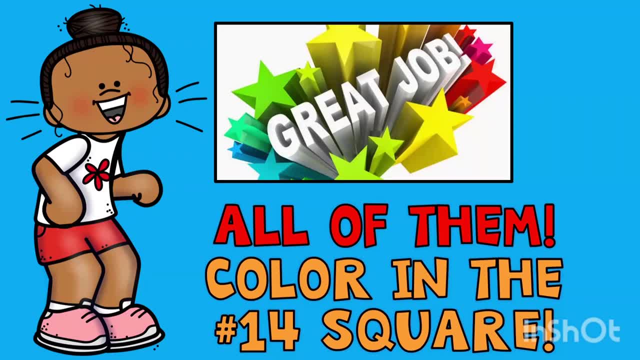 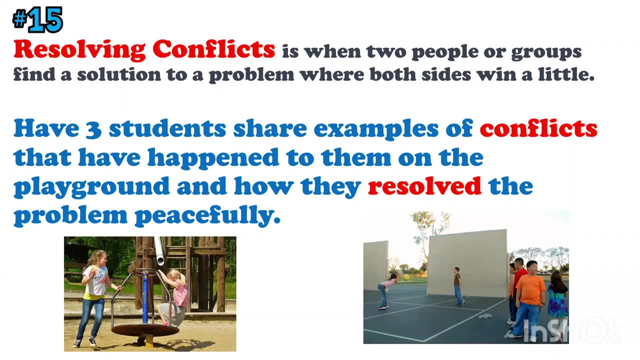 team color in the number 14 square number 15. we're almost there. resolving conflicts is when two people or groups find a solution to a problem where both sides win a little. we might not get what we want all the way, but we get a little bit, especially if we resolve the. 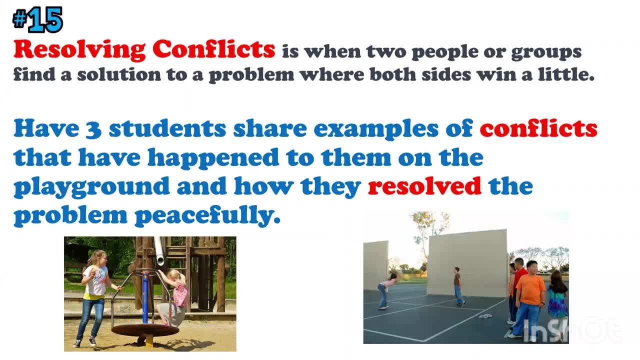 conflict peacefully have three students share examples of conflicts and that they have happened to them on the playground and how they resolved the problem peacefully. pause the game so you can hear all about what conflicts others have solved in your classroom or counseling group. great job. color in the